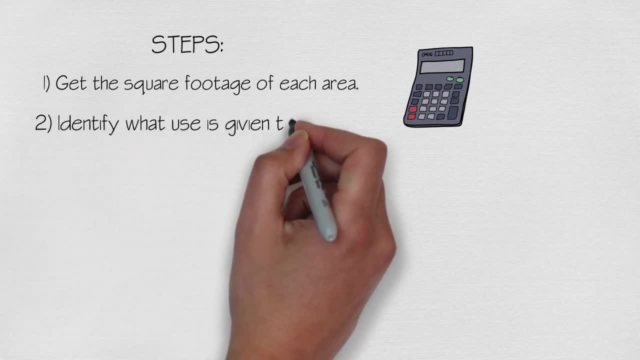 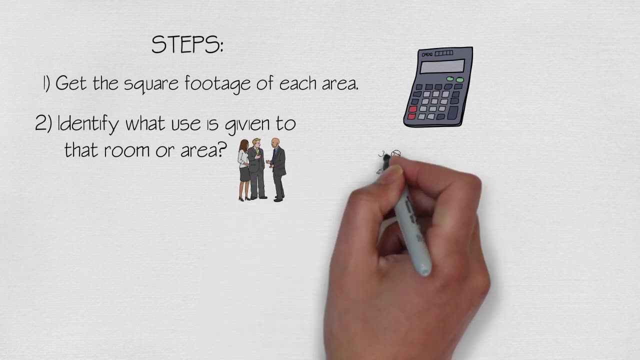 Second, you need to understand and know what use is given to that area or room. For example, it may be an office, a conference room, a break room, a storage room, and these areas are all calculated differently. Once you have the square footage, you need to know how many exits you have in order to know what direction your door needs to swing. You also need to know how many exits you have in order to know what direction your door needs to swing. 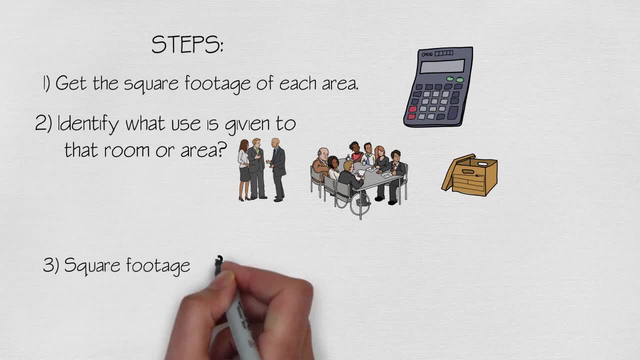 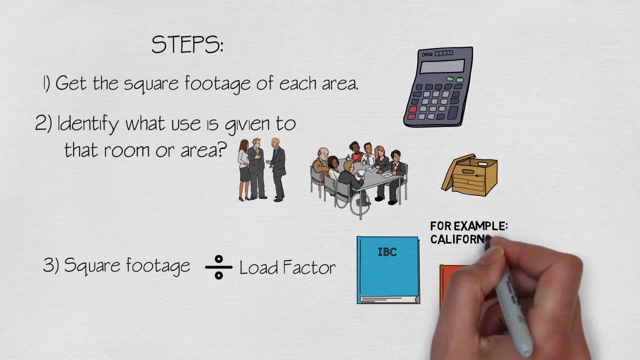 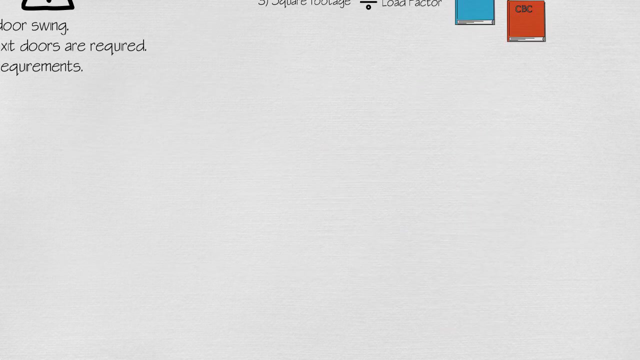 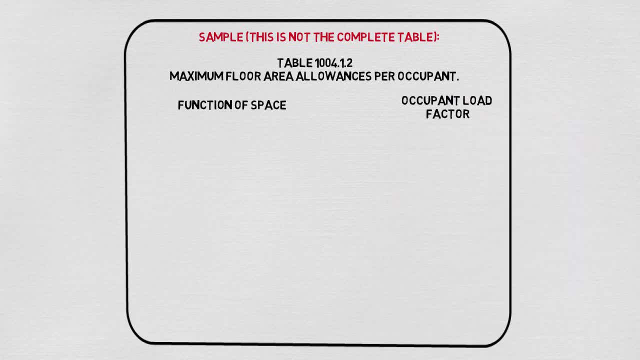 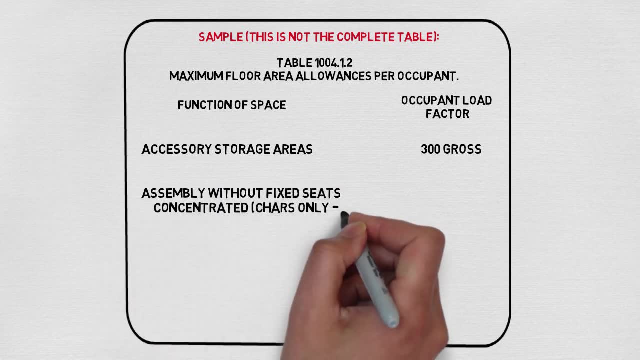 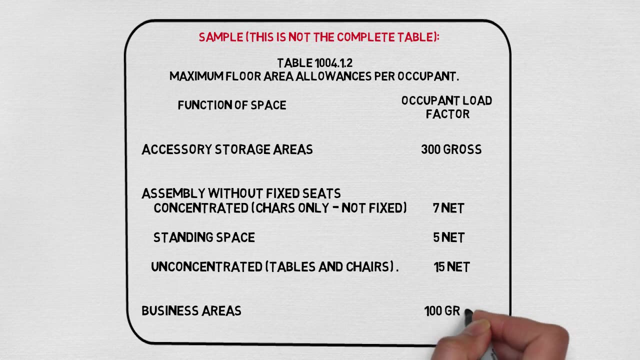 as you look at this table, you will notice that not all room descriptions will be found, so in some instances you're going to have to make a reasonable selection based on the closest matching description. it looks a lot more complicated than it is, but most occupancies are easy to understand. let me show you an example. here we have a typical. 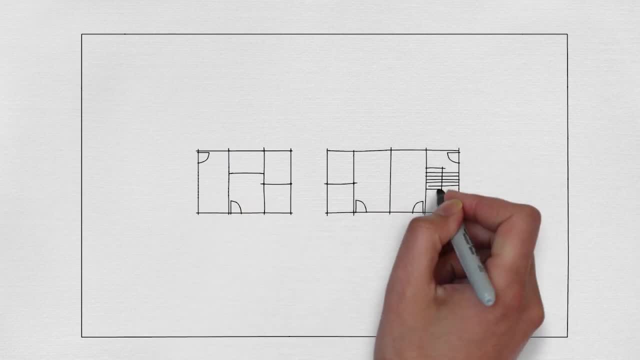 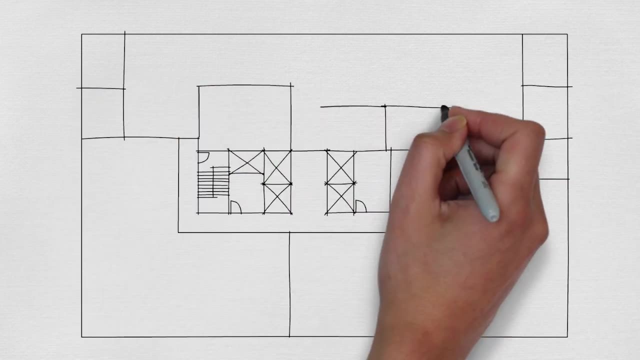 floor plan of an office building and, like many office buildings, the suite we're going to look into only takes a portion of the floor and the rest of the floor is taken by other tenants. therefore, the areas that are shown in red here are the adjacent tenants that are not part of our area. 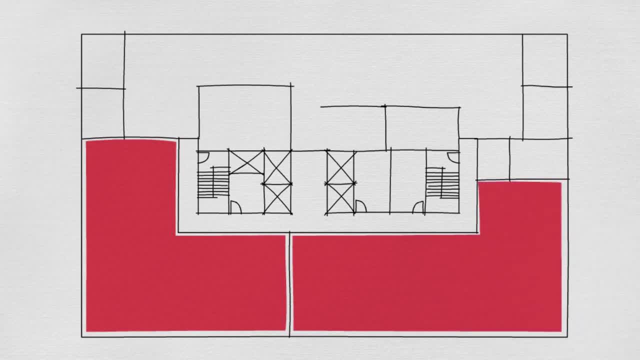 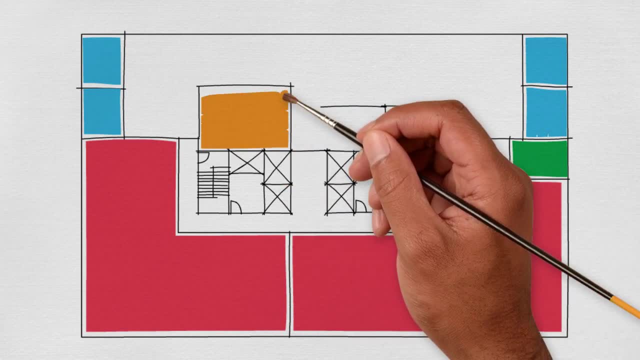 let's assume that our suite is composed of the following: the areas in blue are offices, the area in green is a break room, the areas in orange are conference rooms, the area in purple is a storage room and the rest of the area which is in yellow is 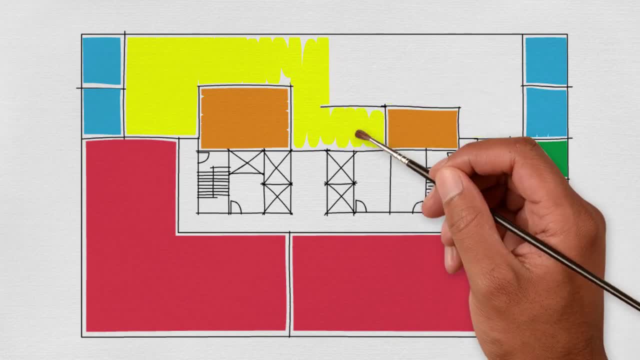 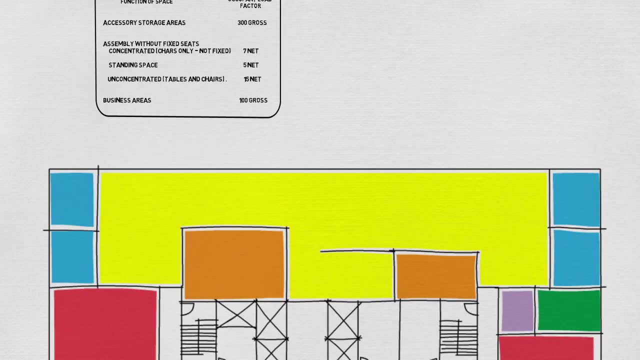 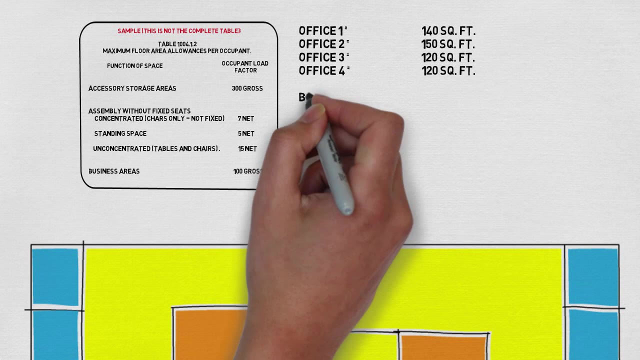 your open office area where you can just use it for cubicles or other open office needs. after you figure this out, now that we know what these areas are being used for, we need to know the square feet of each of these areas. so we tally each one of these areas, we figure out how many square feet. 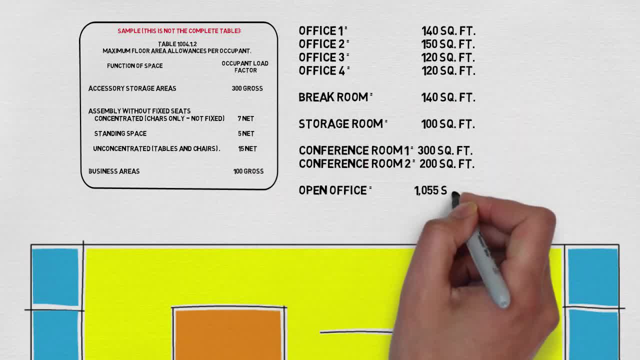 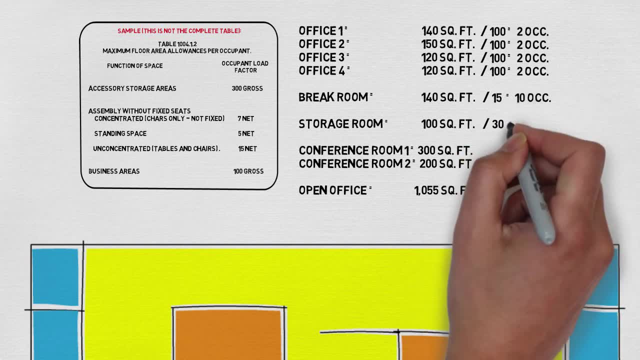 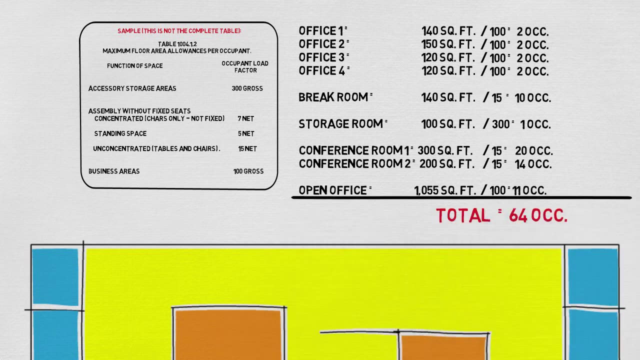 are in each of the offices or each of the break rooms, etc. then we have to divide each square footage by the load factor that is on the table. what this will now give you is the total occupants in your suite. now let's break this down for a minute. as i mentioned earlier, some of these 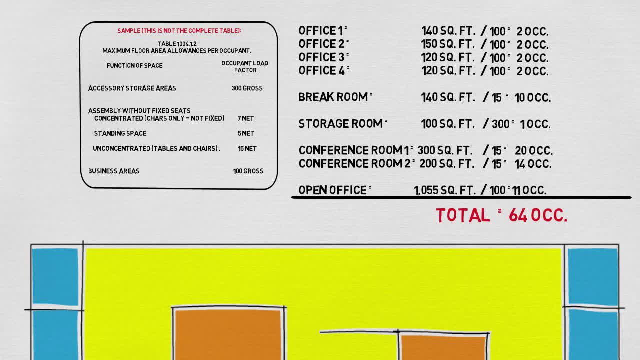 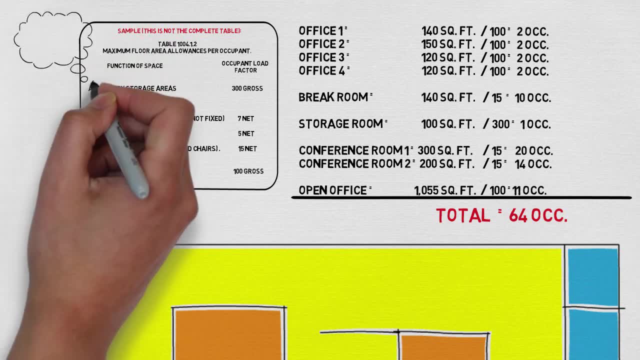 areas are not specifically named in the table in the ibc. let's take a look. the offices, for example. you're not going to find a category called quote-unquote office. instead of the office, you're going to find a category called office. instead of the office, you're going to find a category called office. 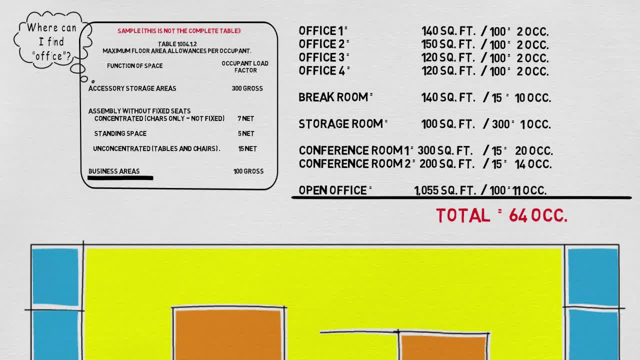 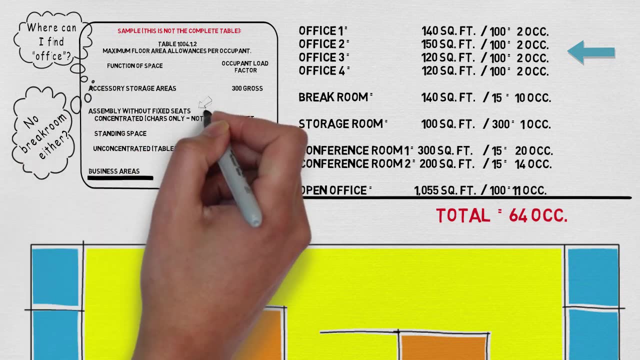 instead, if you look at the table, you'll find a category called business area, and this will let you know that it's one occupant per hundred square feet. you will also not find a place in the table that is called a break room, but in the table you will find a section that's called assembly, without. 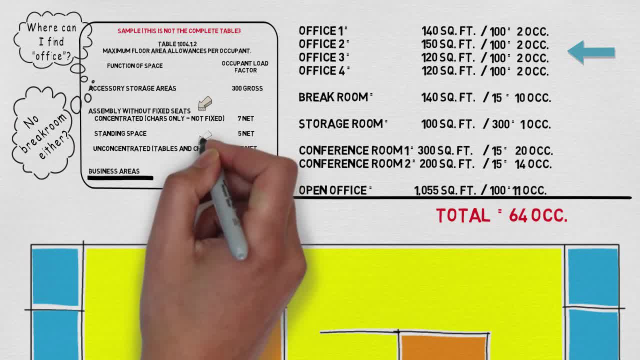 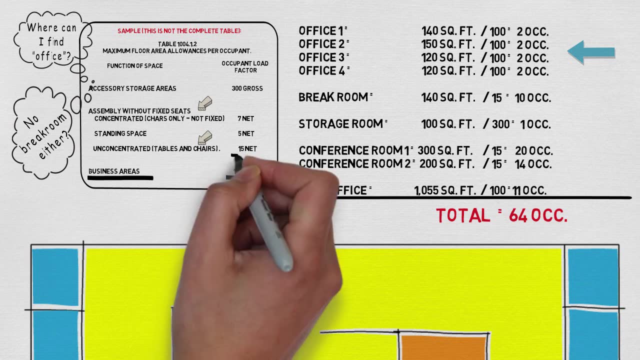 fixed seats. as a matter of fact, underneath that you see a subcategory that's called unconcentrated tables and chairs, and that's what a break room is. you have tables and chairs so that you can eat and have lunch and things like that, and it says there that this will be calculated at one occupant per 15 square feet. 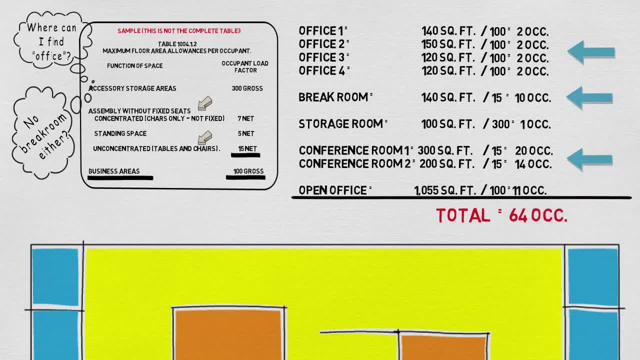 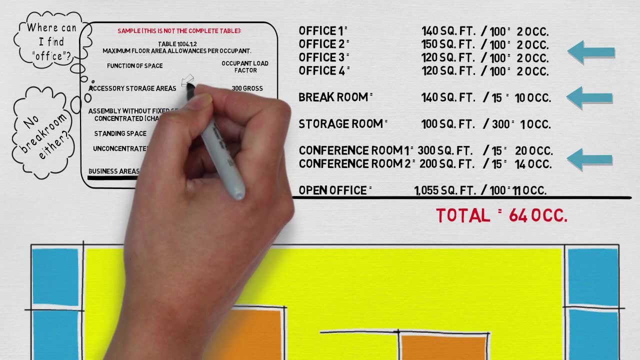 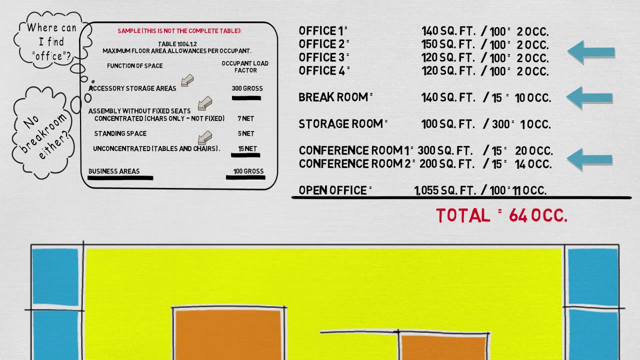 same thing with the conference rooms. a conference room is also used for assembly. you have tables and chairs typically, and so, again, we use an occupancy load of one occupant per every 15 square feet. a storage area is actually noted on the table. there's a category, they're called accessory storage areas, and it lets you know that it's one occupant per. 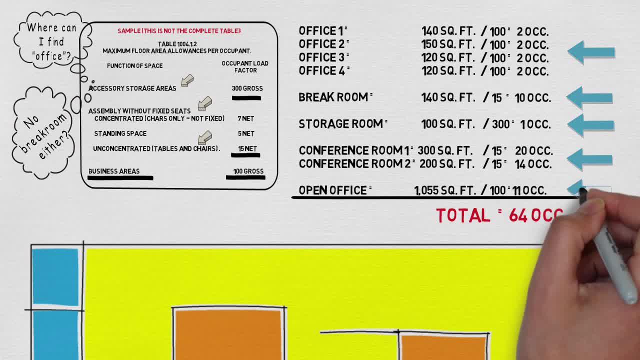 every 300 square feet our open office. well, we already talked about how an office is classified as a business area. so we use one in a hundred square feet. so there you go. that is how you categorize each one of these areas. now let's talk a little bit about the occupants. you will notice 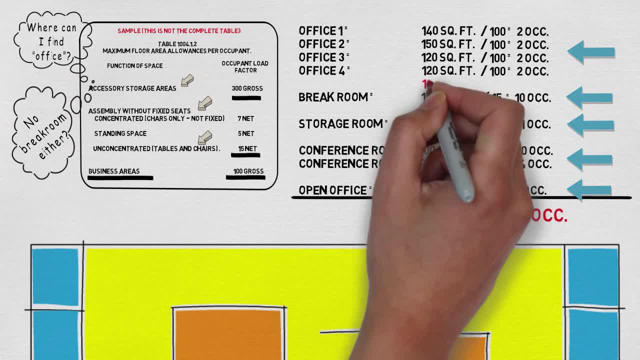 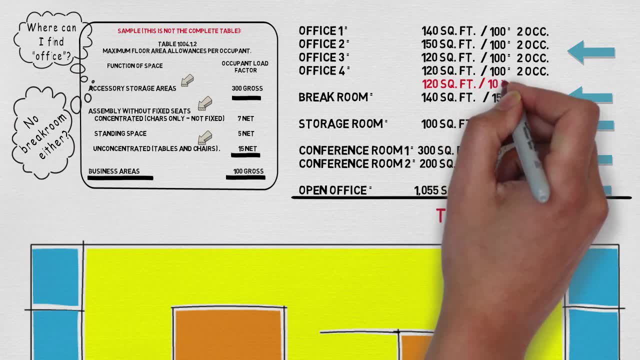 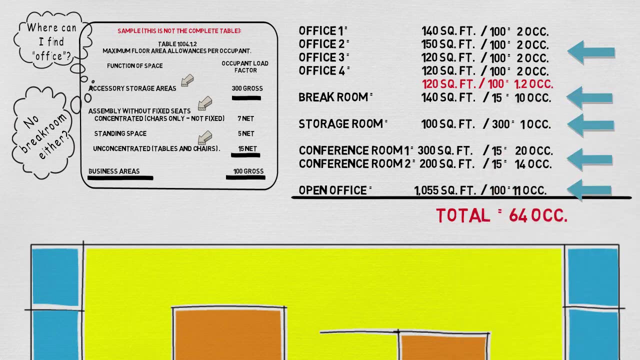 that I rounded up all my occupants. for example, one of the occupants that I'm going to talk about today is a. one of the offices is only 120 square feet. therefore, if you divide 120 square feet by 100, you will only get 1.2 occupants. now you would think that if you're rounding to the nearest hole,